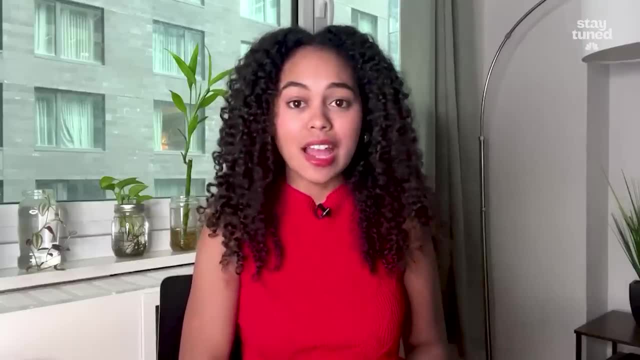 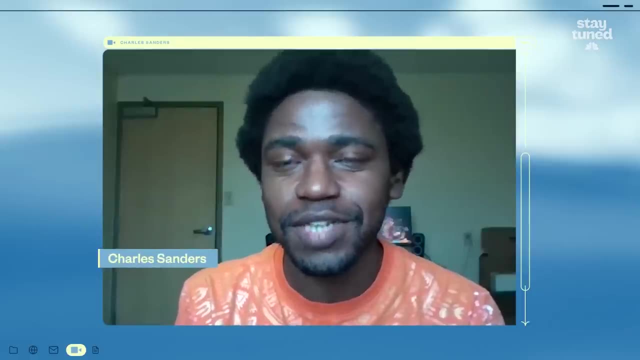 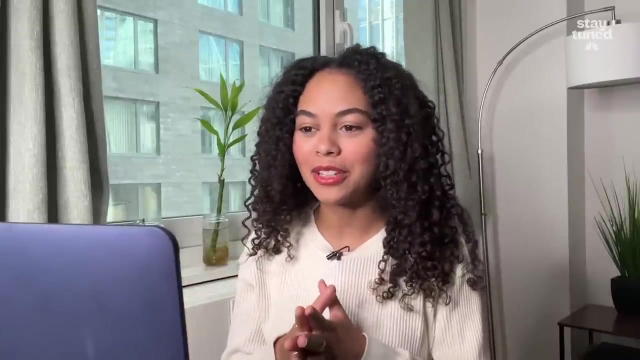 So what's going on here and where are they turning to for guidance? instead? My grandmother was the one that took on that primary responsibility of teaching us all about Christianity. Charles is a grad student at Ohio University. Were there any positive lessons that you took away from Christianity growing up? 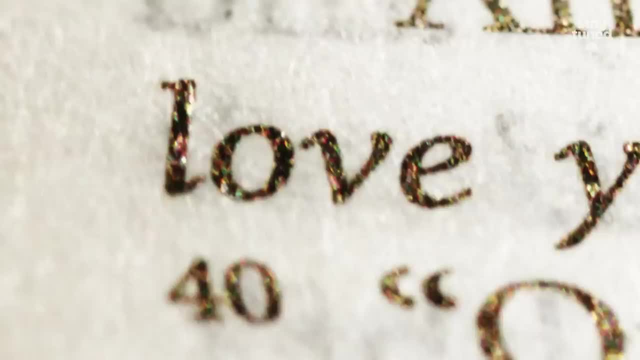 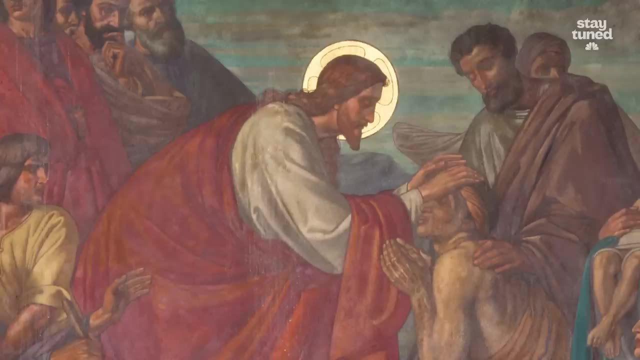 Yeah, Those common ones that you always hear, like love thy neighbor or less like biblical stories that would talk about giving back. I think those are lessons that I got from the church, but you can pretty much get from anywhere and it can apply, no matter what the source is. As I got older, 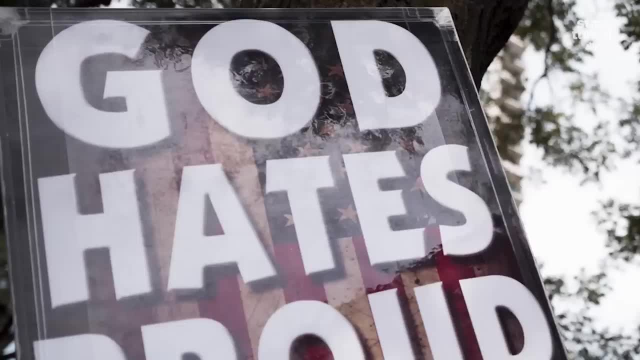 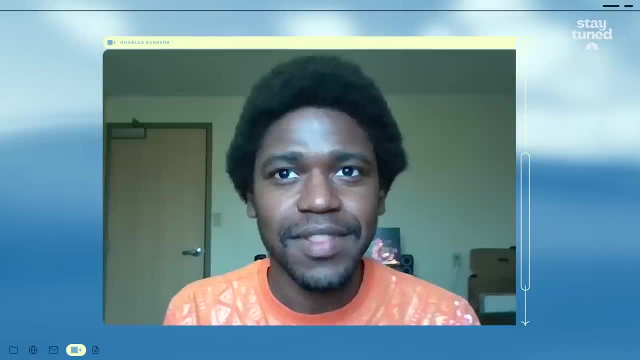 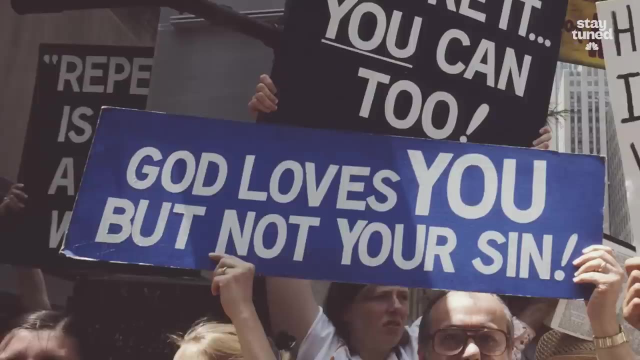 I started to ask more questions about the parts of our religion that didn't necessarily make sense right off the bat to me, And if there was a logical answer then I was willing to accept it. It was those Parts that couldn't necessarily be explained away or were tied to some sort of like hate or 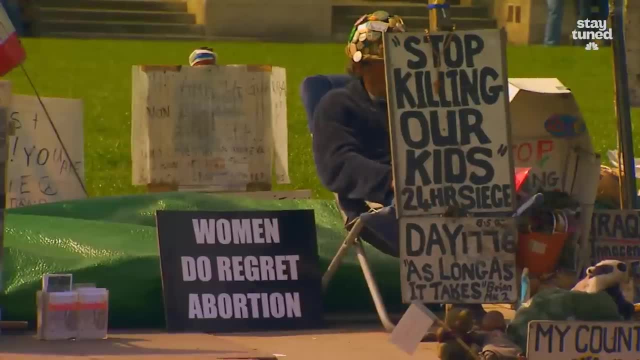 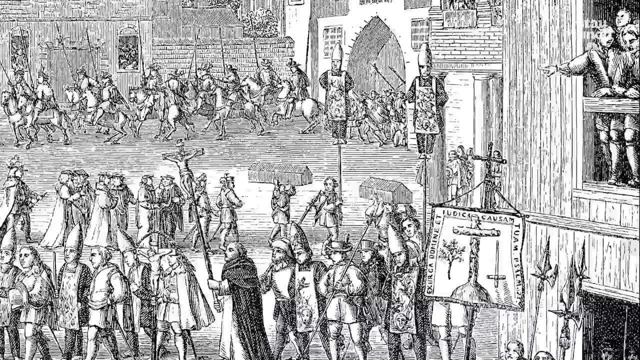 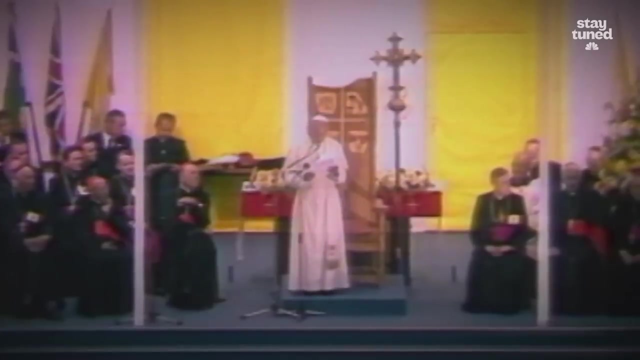 judgment towards others. That's when things started to change. For the last 1700 years, the church was such a cultural and religious and legal dominant force in the lives, especially for those of us in the Western world. Lutheran deacon Ross Murray works with GLAAD. 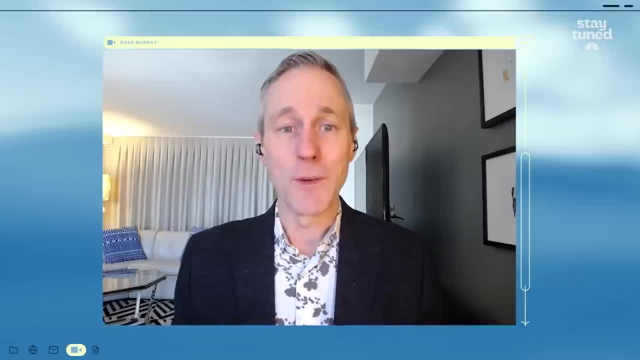 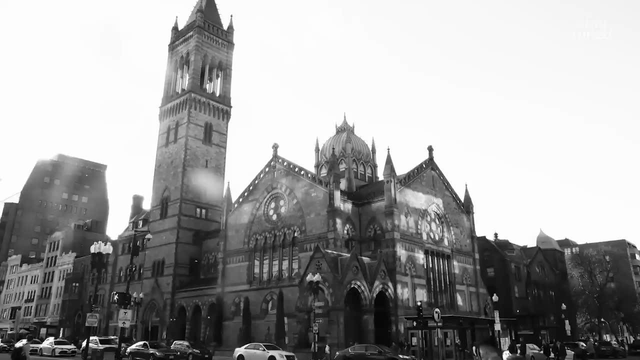 and has been a youth ministry leader for the last 24 years And there's kind of always been this expectation that the church is the center of the town and we will all like come to it. But it's also been a place that has been exclusive. It's kept out. people- LGBTQ people, people of color, people with disabilities, women- And then people realize that they can sometimes get a lot of those spiritual and communal needs met elsewhere and it's not worth the struggle, Even though many areas of Christianity have welcomed everyone in. 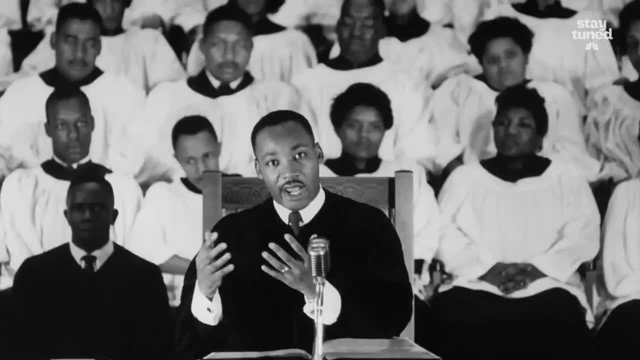 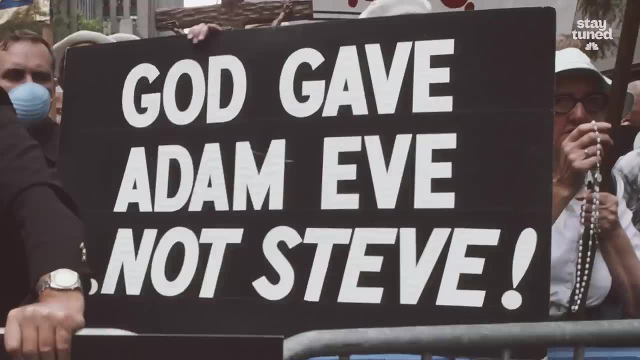 to their pews, served as a place of refuge and revolution and provided thousands of years of guidance and support for millions of people. Ross says that the church has had a complicated history with the queer community from the American colonial period, where men on the Mayflower had to agree. 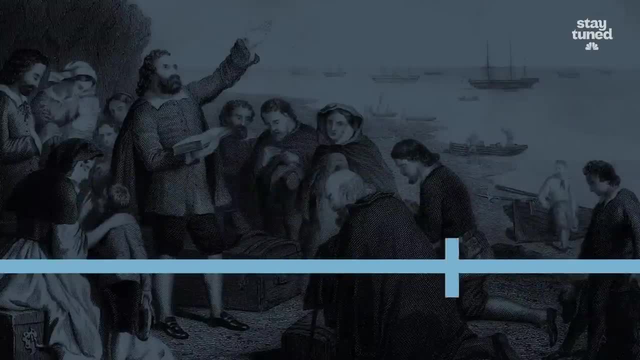 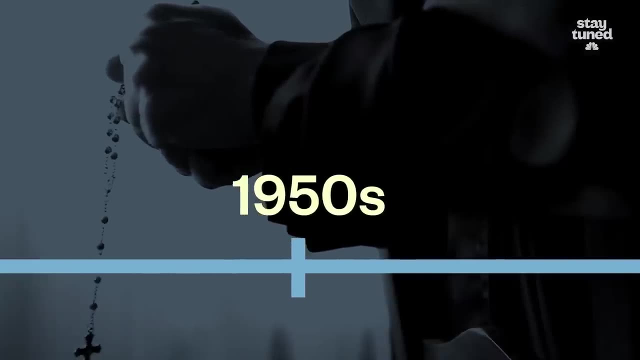 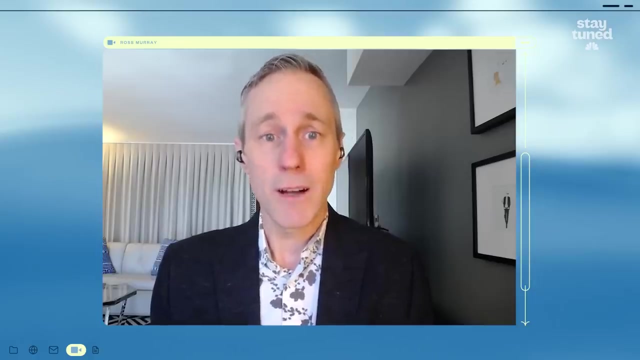 to heterosexual marriages and gender roles through a compact, to the surgical castration of children accused of being homosexual by the church as recent as the 1950s in the Netherlands, and stigma against the gay community During the HIV And AIDS epidemic of the 80s. it is really hard to give up power and privilege, And we, as the church, 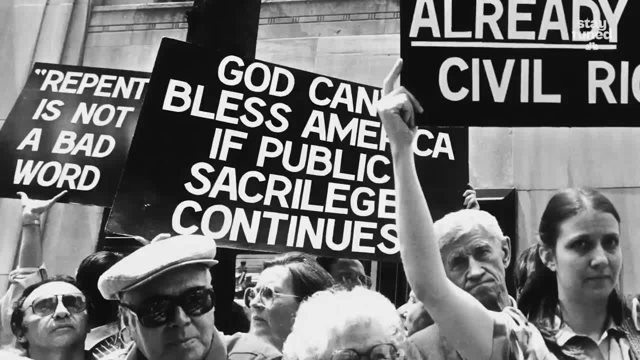 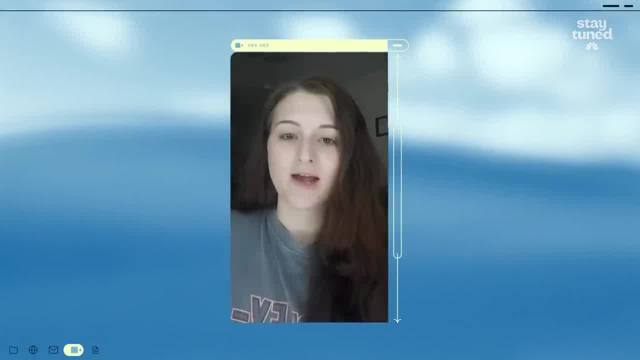 have been able to have that power and privilege for a long time And giving that up or sharing it with other groups feels like a loss, feels like an attack. I really hate how the church made me feel about the LGBTQ community and that I had to look down on people like that- And I actually had. 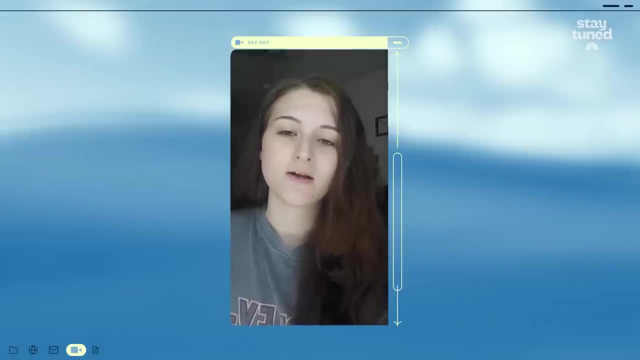 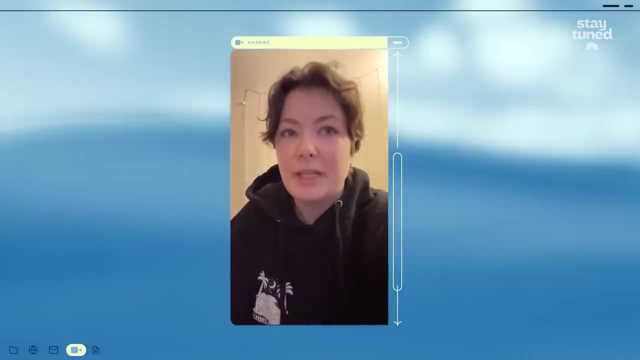 friends who would not tell me that They were in that community because of fear that I would no longer want to be their friends. It started to become a very negative environment. It felt like everything was a sin. It's a sin to be gay or like you can't love who you love. 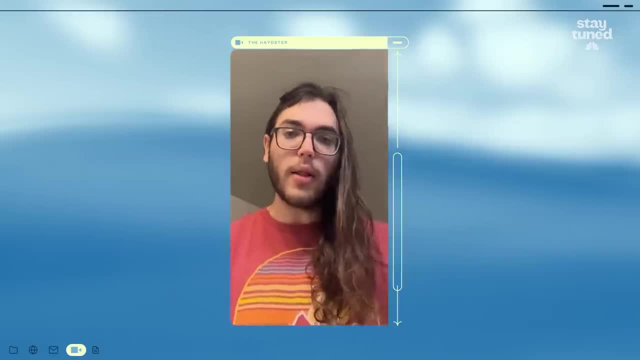 And that's really harmful. My father's a pastor. I think that a lot of Gen Z hears the Bible and sees Jesus as a good role model, but then sees the church not living up to his example. i identify as bisexual. honestly, didn't come to terms with 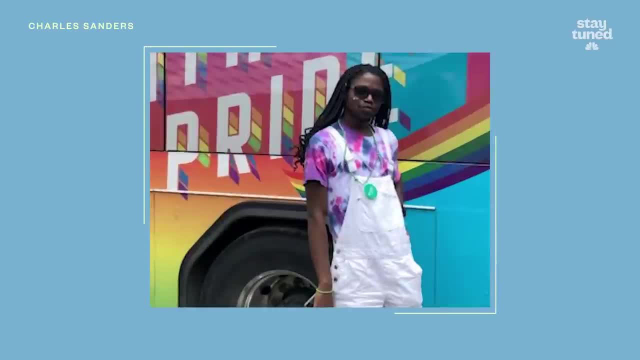 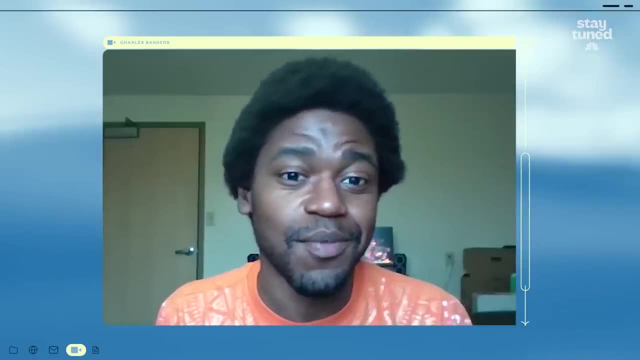 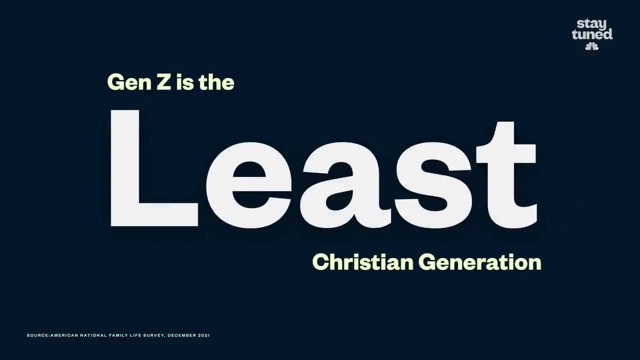 until very recently because i was struggling back and forth with: okay, this is who i am, this is how i feel, but is that me like completely going against, like this thing that i've known basically since birth? in a recent survey, more than a third of gen z identify as non-religious. in fact, gen z is the 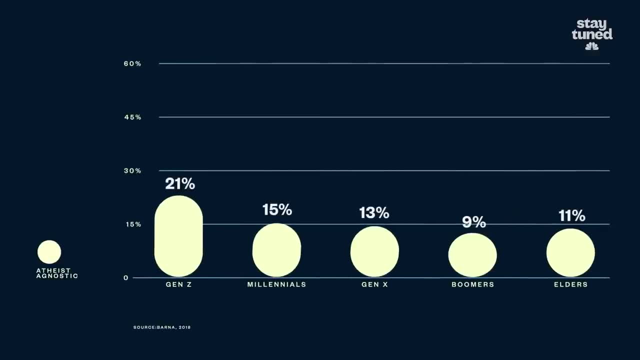 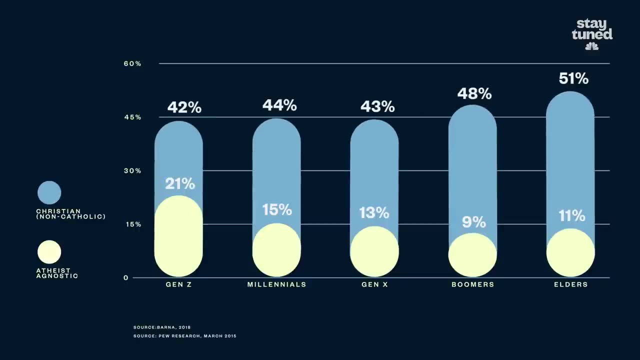 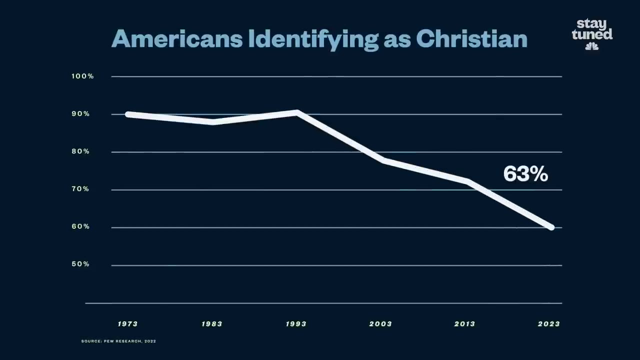 least christian generation, being most likely to identify as atheist or agnostic than any other generation. but this didn't start with gen z. each generation following the silent generation has been getting less and less christian. in 2020, over 60 percent of americans identified as christian. 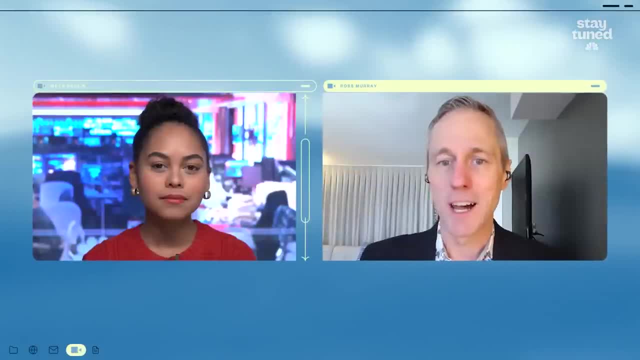 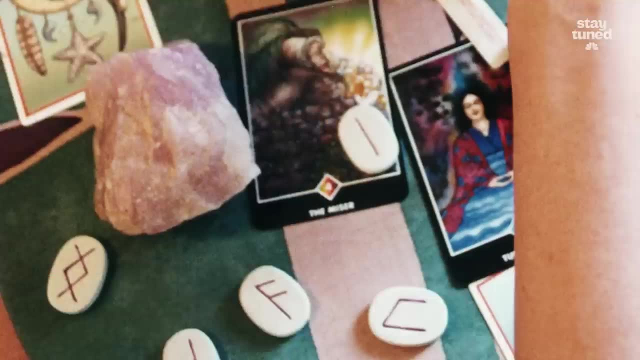 down from 90 percent 50 years ago. i think, as time has gone on, people are very much less invested in the institution of the church. they still have a really strong sense of spirituality and wanting that form of connection, but they're often looking for that in. 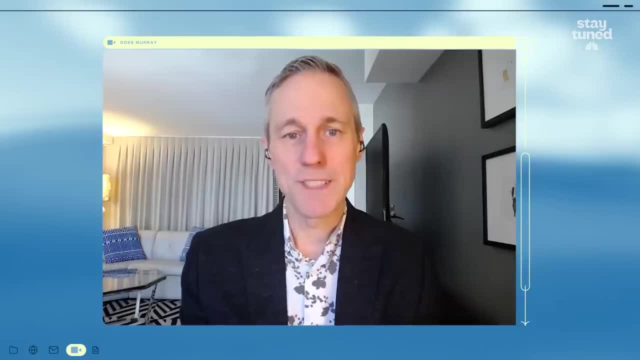 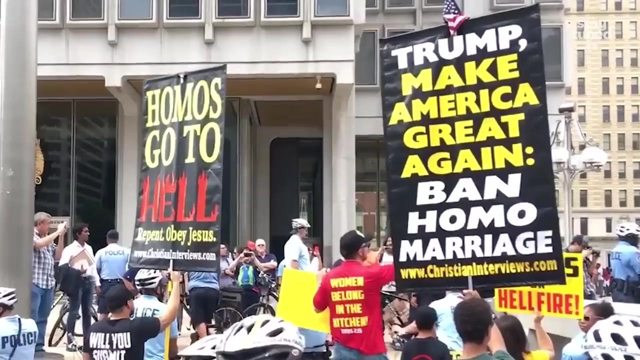 their lives, and i think that's what's happening in the church right now. we've seen a long version of using religion as not a nurturing thing, but actually as a weapon, right, or as a way to harm others, and i think that's what people are really, really tired of confronted with.